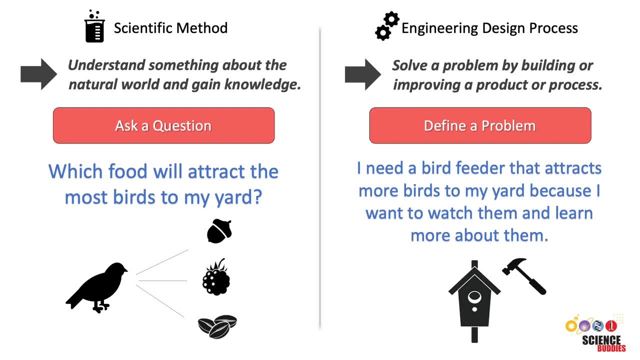 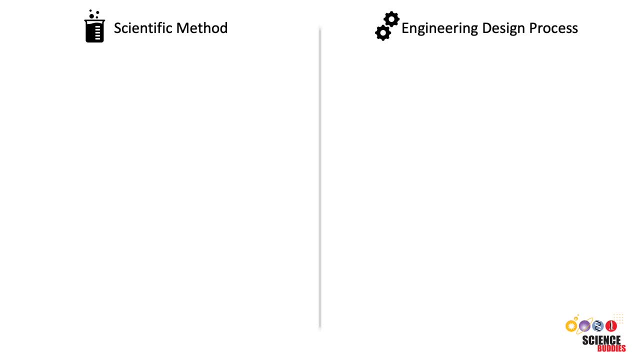 I need a bird feeder that attracts more birds to my yard because I want to watch them and learn more about them. The second step for both the scientific method and the engineering design process is to do background research. In our scientific method example, we might research what different types of foods birds eat or what other scientists have found out. 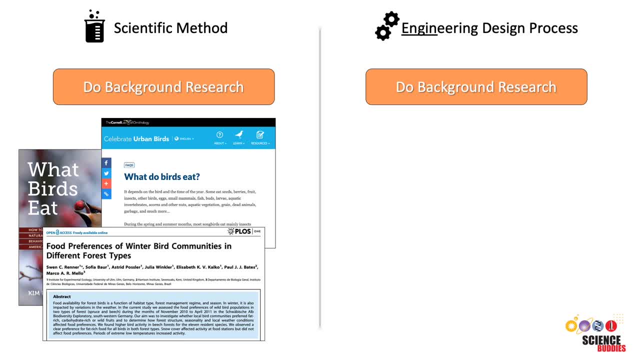 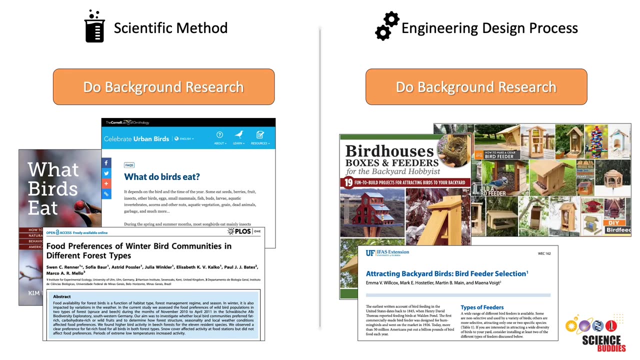 about birds food preferences In our engineering design process. example, our research might focus on finding out how other engineers have approached building a bird feeder, what challenges they have encountered, or what types of bird feeders already exist and what types of birds use them. The next: 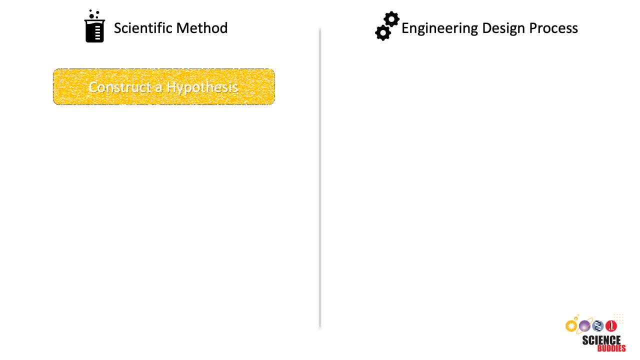 step when using the scientific method is to make a hypothesis or educated guess about how we think our question will be answered by our experiment In our bird watching project. maybe our background research revealed that birds enjoy sweet foods. We might hypothesize that if we put blueberries, sunflower seeds, a seed 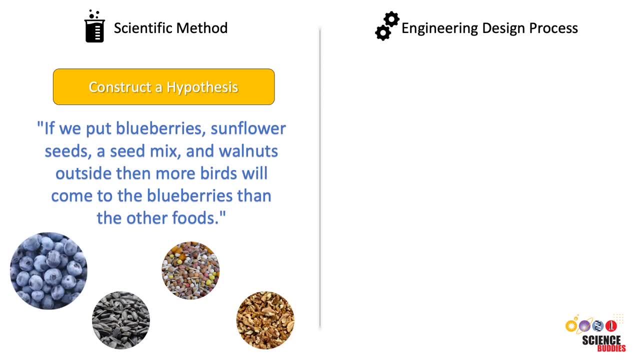 mix and walnuts outside, then more birds will come to the blueberries than the other foods, because they are sweet and juicy. When using the engineering design process, we won't make a hypothesis. Instead, the next step is to specify the criteria or requirements for our product or solution. When building a 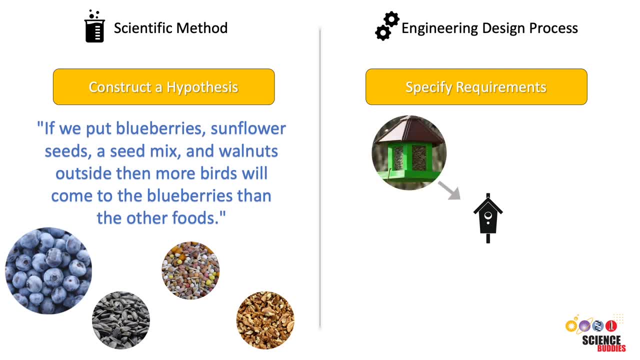 bird feeder, for example. we would need to make it big enough and sturdy enough to hold a certain amount of bird food. It should be weatherproof, safe for the birds, keep away squirrels and be relatively inexpensive and easy to build. 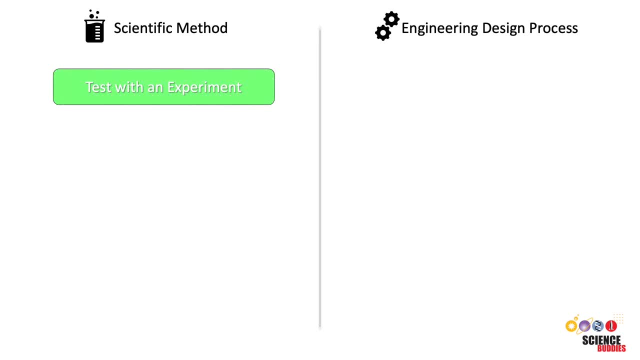 When following the scientific method, we will test our hypothesis by designing and carrying it. To do this, we first need to identify the variables of the experiment. Then we come up with an experimental procedure that will allow us to collect data about the birds' food preferences, For example. we could put out several identical 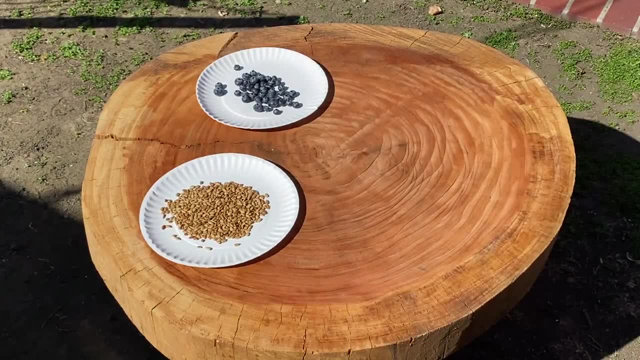 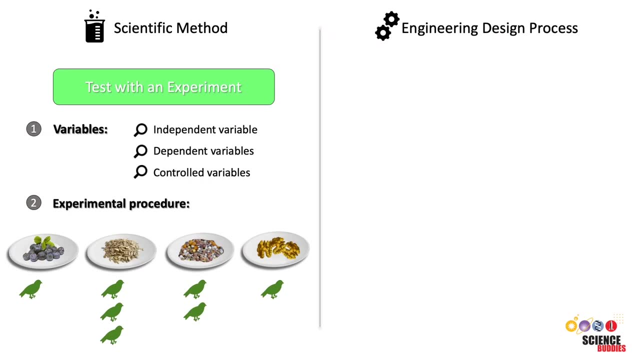 containers that each contain a different type of food and then collect data about the number of birds that visit each container or record how quickly the food in each container empties. When following the engineering design process, we won't do the same kind of experiment. Instead, we continue brainstorming solutions to 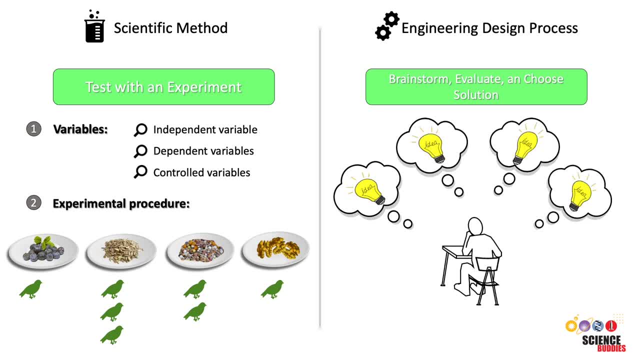 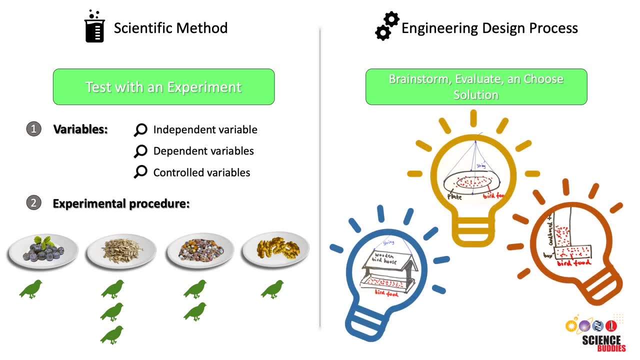 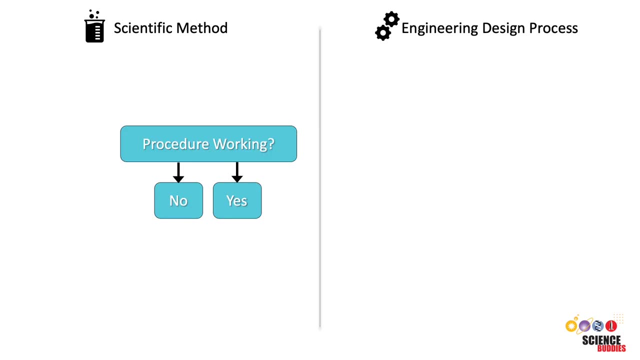 our problem: evaluating the different solutions and choosing the best one to try first For our project. this means we would brainstorm different bird feeder designs and decide which one we will build first. In the scientific method we need to actively ask: is the procedure working as we experiment and collect? 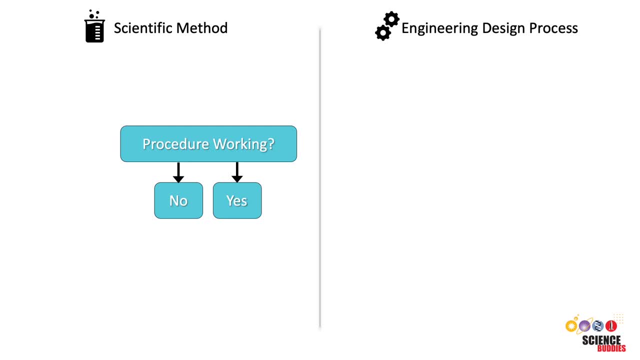 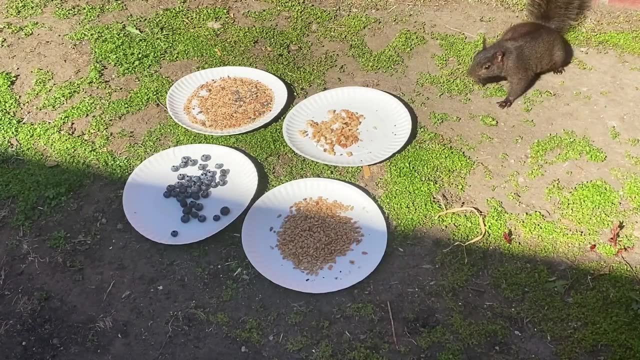 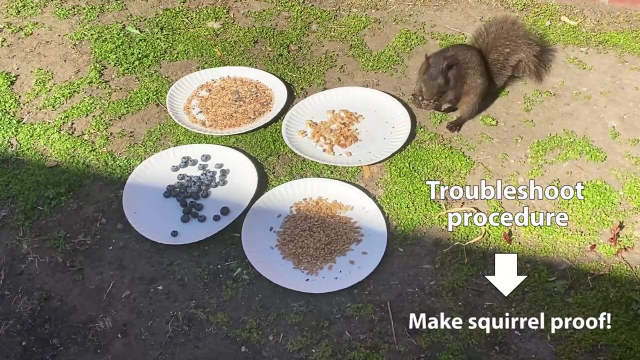 data. If the experiment is not working, we will need to troubleshoot the procedure and restart the experiment. For example, we might find that other animals besides birds eat the food we put out, which means that we will have to rethink our procedure and then redo the experiment. The goal of conducting the experiment is to collect enough 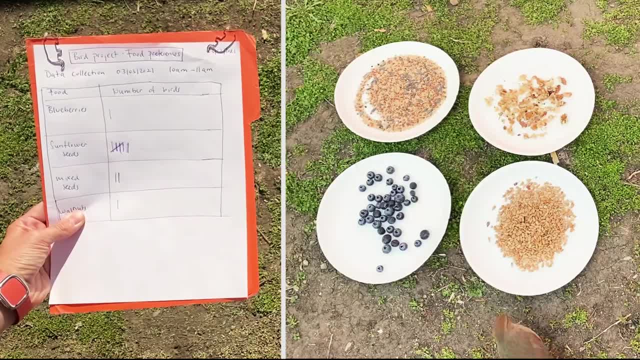 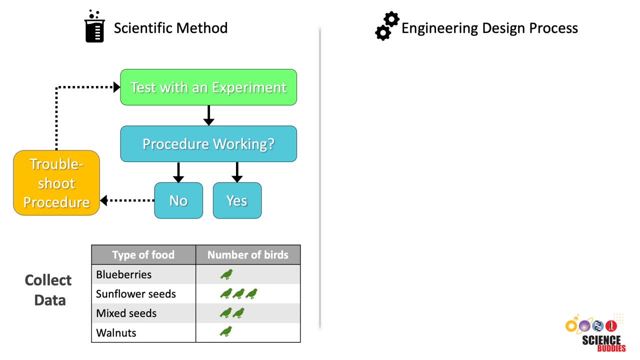 data to confidently determine if our hypothesis is being supported or not. In the engineering design process, after deciding which bird feeder design we want to try first, the next step is developing and building a prototype. This means we use our previous sketches or drawings of the 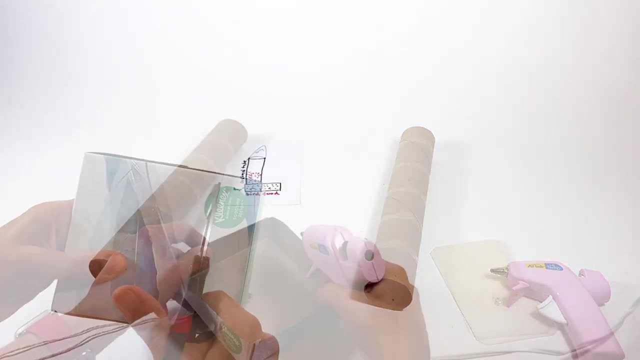 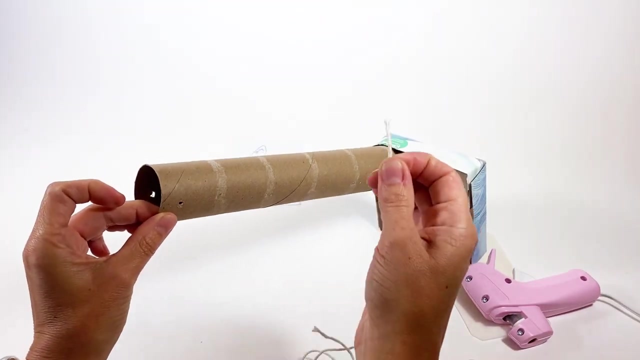 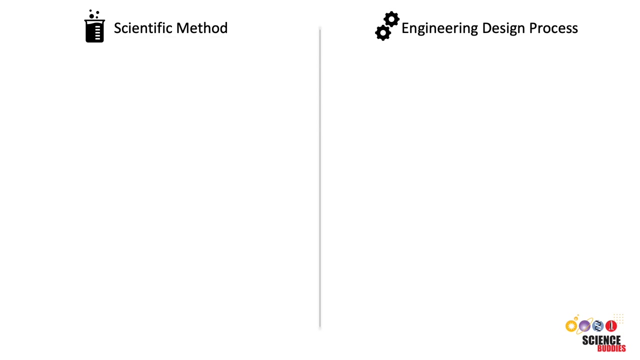 bird feeder we want to build, choose the materials for each part of the design and then build our first bird feeder prototype. We know we might need to make changes later. Our prototype is just an initial build that will let us begin testing our product In the scientific method after we finish. 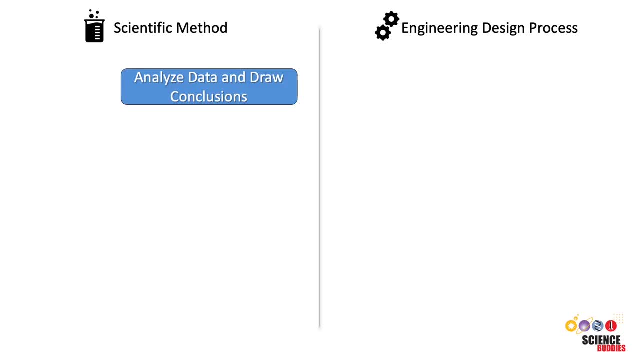 our procedure and have collected our data. we review and analyze the data. This includes making graphs and evaluating if the data is correct. We then review and analyze the data. This includes making sure if the collected data is complete, of good enough quality and is valid. If our data is. 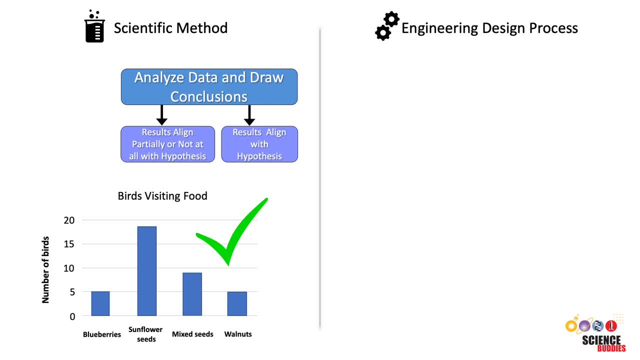 sufficient. we can then draw conclusions about whether or not our data supports our hypothesis. Sometimes, the data leads to more questions and the process starts again with a slightly different question and a new hypothesis. The next step in the engineering design process is testing our prototype, which involves measuring the prototype's performance as well as evaluating. 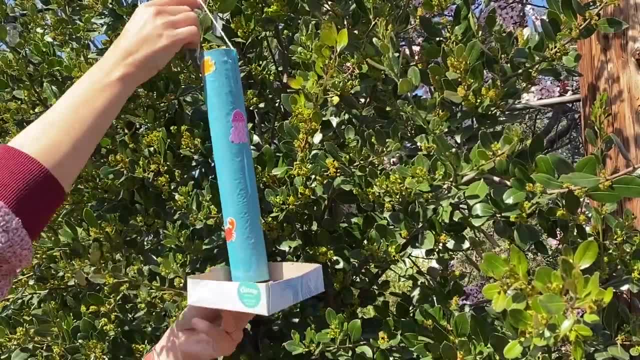 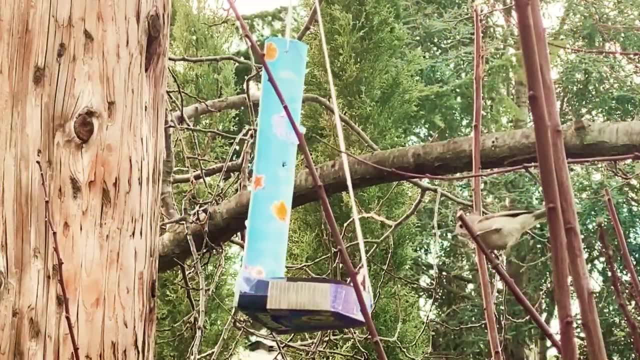 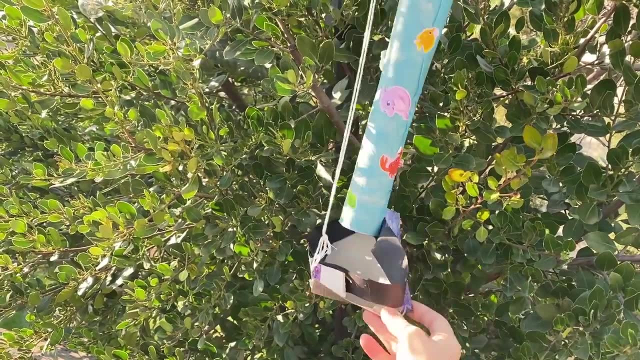 it against our design criteria For our bird feeder. this means we could observe how well birds interact with our prototype and keep track of metrics like how many birds visit the feeder, how many eat from the feeder, whether squirrels get to the food and whether any parts of the bird feeder get damaged. If we find